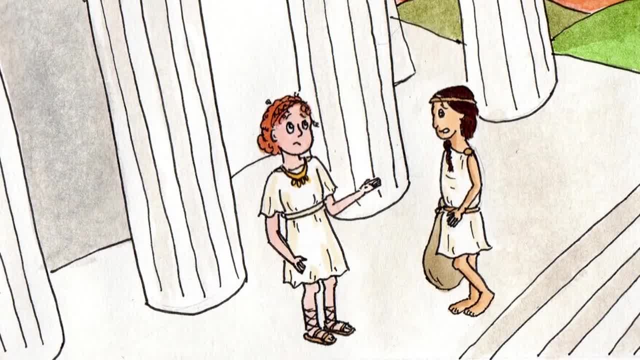 Um, I'm very sorry, obviously, but what do you need me for? Delphi looked at Delphi. Delphi looked at her as though it was the most obvious thing in the world. Well, you work in the temples, don't you? 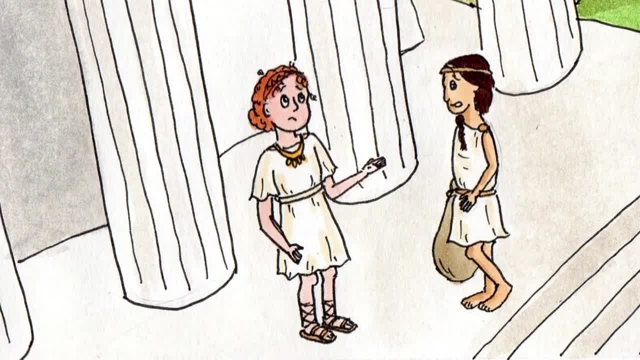 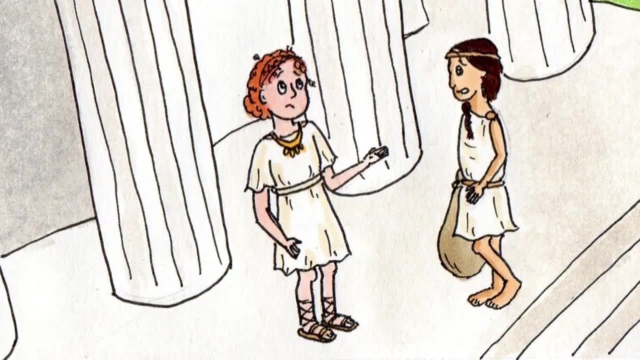 Mertis frowned Well sort of. I was chosen to be an attendant to the goddess, she replied. Mertis was from a richer family than Delphi and had been specially chosen to spend a year in the Parthenon in service to Aphrodite. It was seen to be quite an honour. 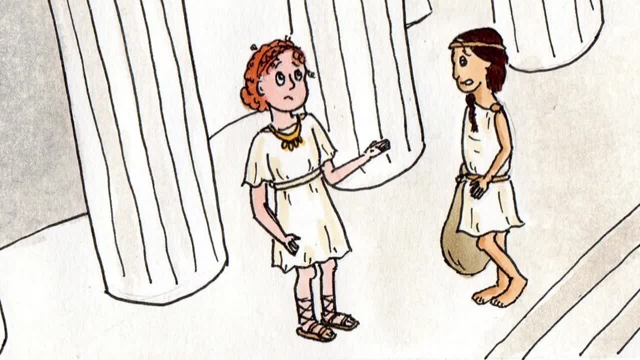 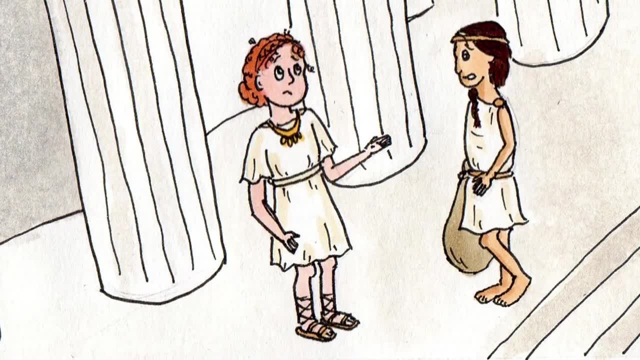 Delphi had not been chosen, but then she never thought she would be. Whatever, Can I sleep in the temple tonight, Please, Mertis? I don't know what else to do. Mertis bit her lip nervously. This was actually quite a common request. 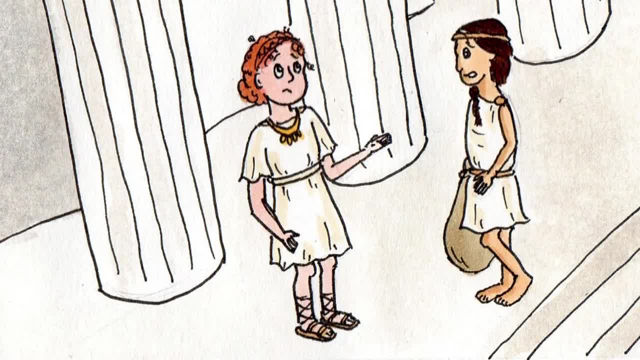 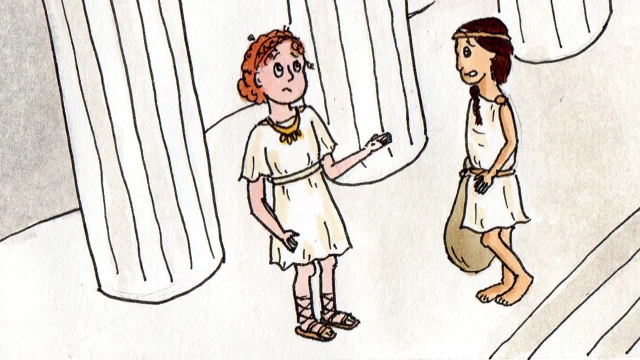 Greeks believed that the dreams you have at night were messages from the gods. So if you wanted help from the gods, you slept in a temple and hoped you got a useful dream. This did not always work. Please, I'll stay really quiet, I promise. Delphi pleaded. 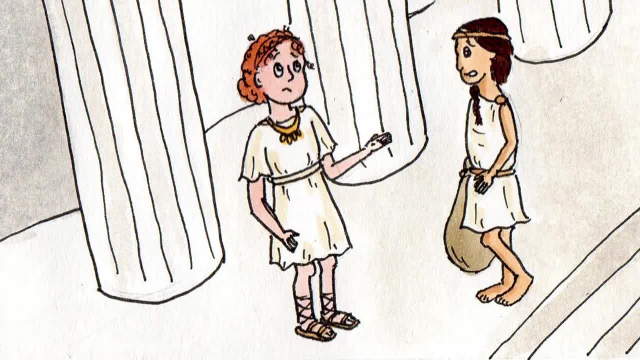 Mertis sighed. There was something about Delphi that always made her nervous. Um, okay, You just have to sleep on the floor though. That's okay, I brought some blankets. Thanks, Mertis. Oh, you won. 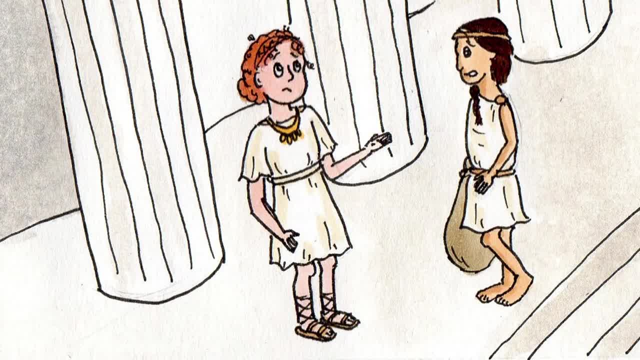 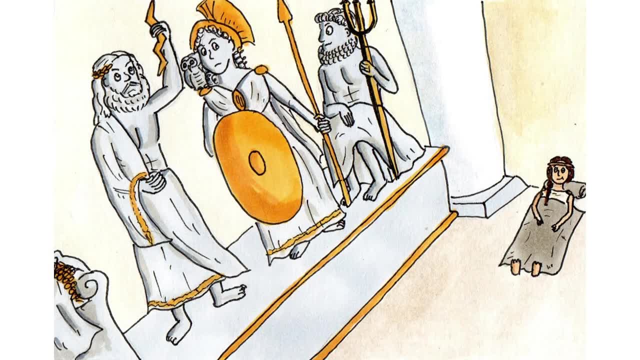 Mertis pointed out a corner just inside the entrance, smiled at her in a rather scared way and scuttled back inside the temple. Delphi spread out her blanket on the marble floor and bunched up another one for a pillow. She lay down and groaned. This was not going to be a comfortable night. She stared up at the ceiling. 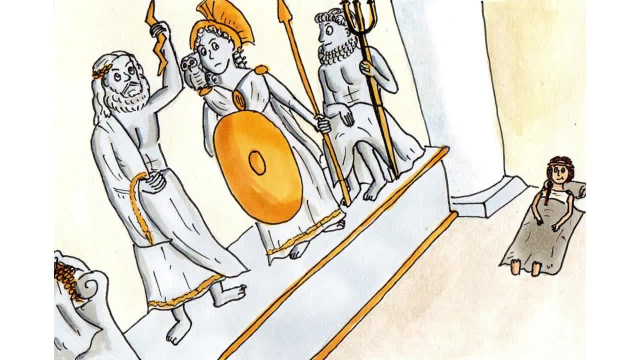 By the last rays of sunlight, she could make out the painted sculptures and pictures which decorated the inside of the Parthenon. There were some of the most spectacular in the city. They showed the gods doing what they do best: posing. There was Zeus, the ruler of the gods, with his white beard and thunderbolts. Next to him was Athena. 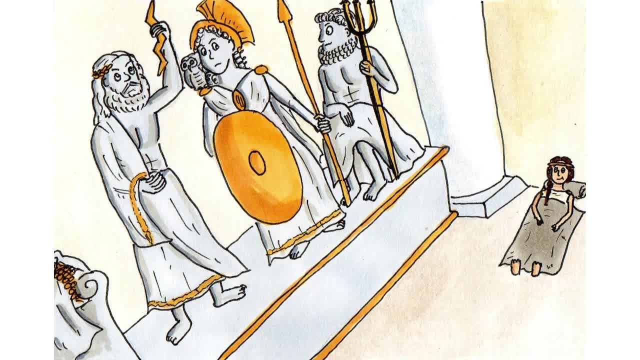 was Athena, the goddess of the city, carrying her golden shield and spear and wearing a golden helmet. She could even see Dionysus, who was looking as dopey as ever. They were almost countless in number and each was glorious and powerful. They spread out above her like stars. 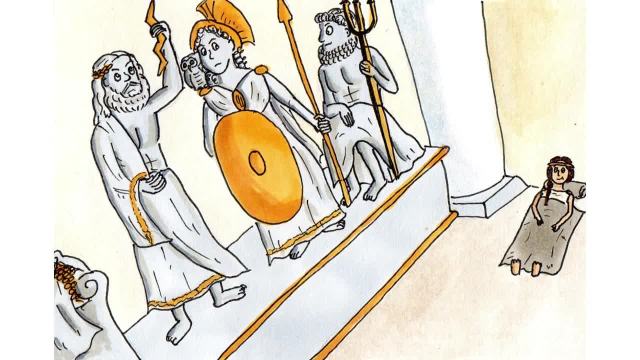 in the sky. Delphi closed her eyes. She so wanted Socrates to be free. She felt like she had learned so much from him already and they had barely spoken. Imagine if he could be her teacher. But this was a long shot. she knew She had heard of people sleeping in the temples. to speak to the 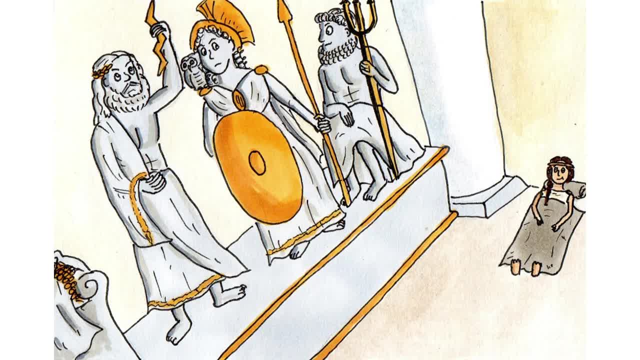 gods, but had always doubted if it really worked. However, she had already spoken to a god recently, so maybe they would speak to her again. And if anyone knew about freedom, then it was the gods. They must be free to do anything, she thought. Who could be more free to do something than a god? 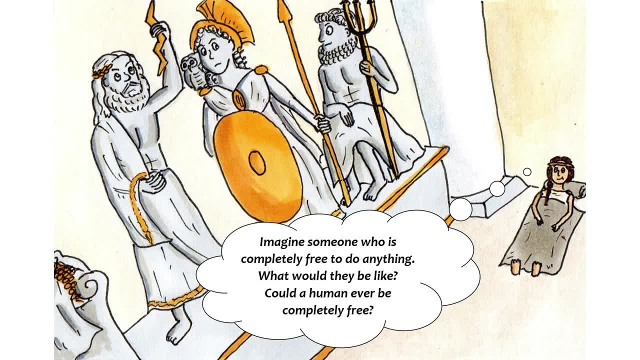 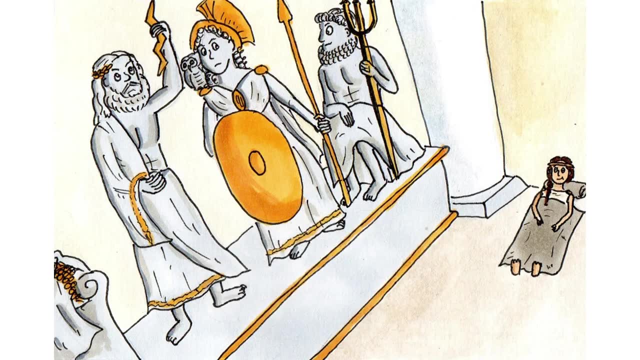 Imagine someone who is completely free to do anything. What would they be like? Could a human ever be completely free? When Delphi woke up, she was rather confused. Where was her bedroom? The ceiling looked different. It was sky Up. you get, then, and let's have a look at you. 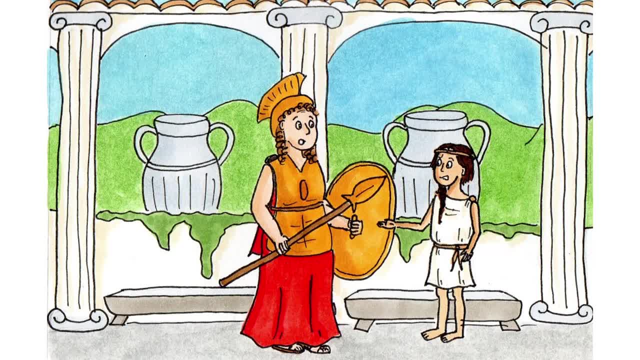 Delphi leapt to her feet and her eyes widened. In front of her was a middle-aged and rather dumpy woman dressed in red cloth and shining armour that didn't quite fit any more. She was carrying a golden shield and spear and was wearing a golden helmet. Delphi's eyes were 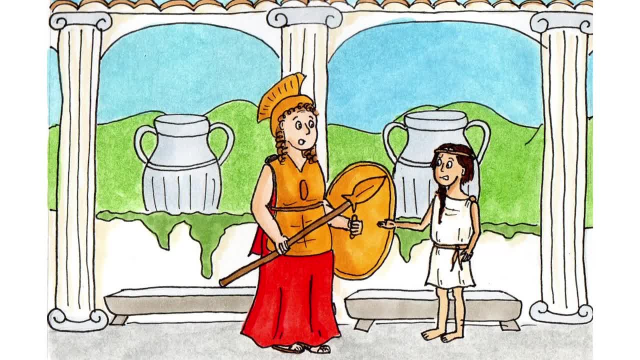 widened. Are you Athena, goddess of wisdom? Athens and owls: I'm quite happy with the first two things, but the owl droppings do get a bit tiresome after a while. Nice to meet you, dear Delphi, gaped at her. 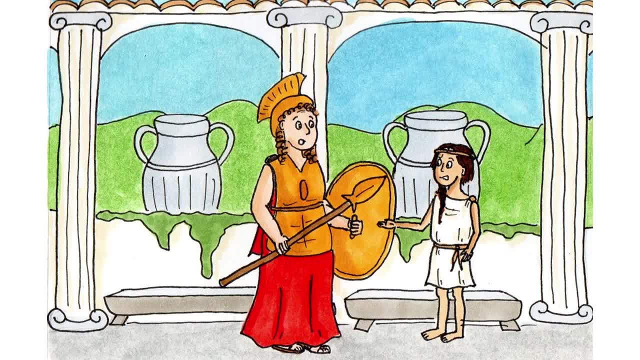 Well, don't just stand there like a fish, said the woman. Come along now. Athena started to lead her across the hallway. Delphi wasn't sure where she was. It still looked a bit like the Parthenon, but was open to the sky and much bigger. There were lots of fountains and 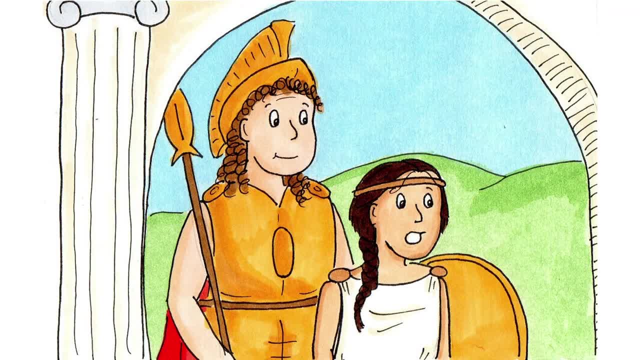 pot plants around. Um, where am I? Delphi asked. Where do you think you are? my dear Athena replied: You fell asleep in my temple and now you're talking to me, so you must be. She paused like a schoolteacher, letting Delphi finish. 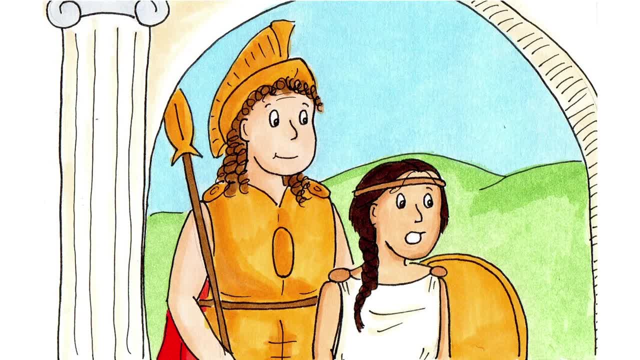 On Olympus, Delphi whispered: The home of the gods. Bingo snapped Athena. Although she could recognise her, Athena wasn't quite what Delphi had expected. The statues at home were all of someone a lot younger for one thing, Through here, dear, that's it. I expect you want to talk to Zeus about Socrates, don't you? 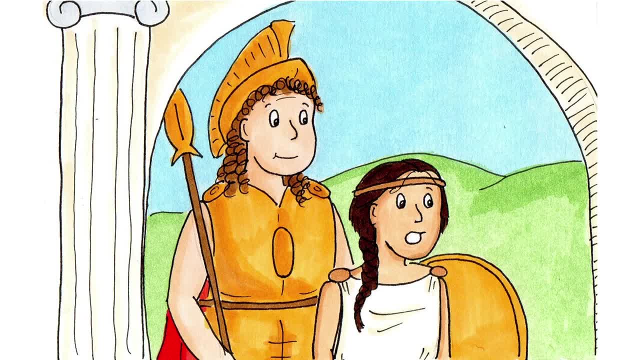 Athena led Delphi towards the stone archway. How did you know, Goddess of wisdom? as I said, Come on, don't dilly-dally. Delphi had to almost run to keep up with her When they went through the archway and into. 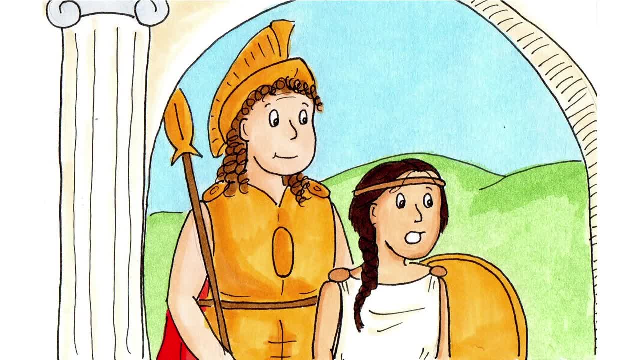 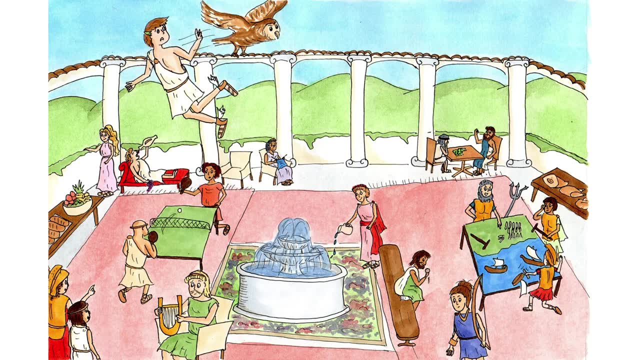 the large courtyard beyond Delphi's brain almost refused to take it all in. The courtyard was enormous but furnished with a huge range of comfy-looking armchairs. There were thick carpets of a deep red colour on the marble floors and enormous amounts of food. 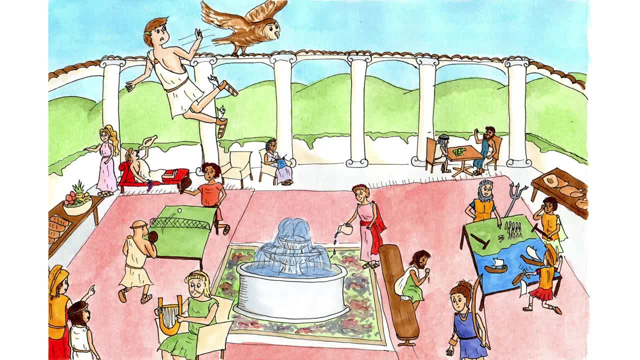 piled high on tables And all the gods were there. Some of them were relaxing in chairs or having a drink. Others were sat at tables with jigsaws, What looked like board games. Two of them were playing table tennis. Time for some quick introductions, I think, said Athena marching Delphi through the assembled gods. 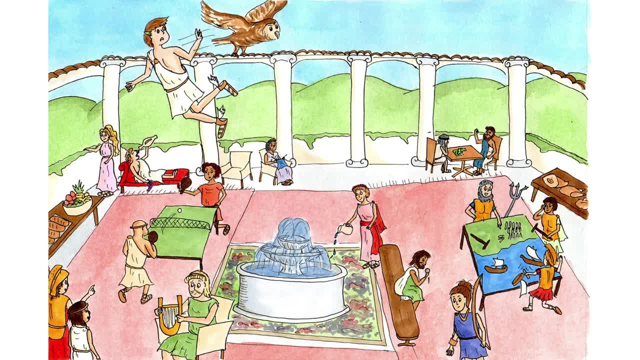 and goddesses That's Apollo making that awful racket. Delphi looked to see a blonde and rather confused-looking man concentrating on a small golden harp. He was attempting, and broadly failing, to play a tune from a papyrus book called Simple Harp Tunes, Volume 2.. 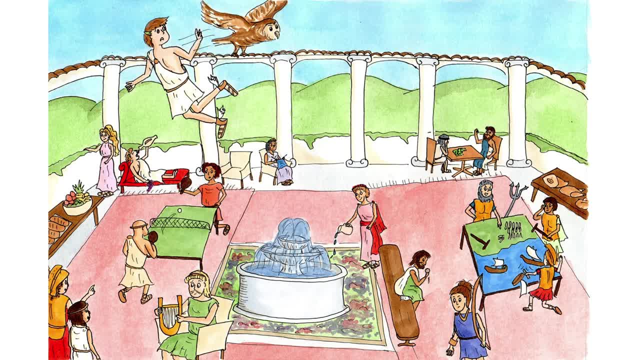 And up there is Hermes the messenger. god, A brown-haired young man was hovering above them, wearing shoes with tiny wings attached. He gave them a wave: Don't ask if you can have a go with them. He never was much good at sharing. 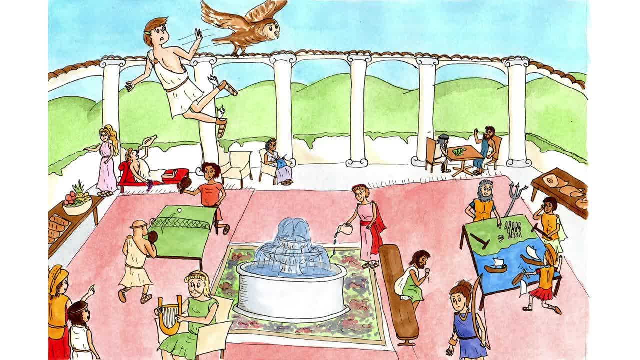 Delphi waved back. Who else is there? Let's see. That's Demeter watering the plants and Hera with the knitting, And the boys over there that's Ares, Poseidon and Hef. Delphi looked over to the table to see three men in armour playing with what looked like toy. 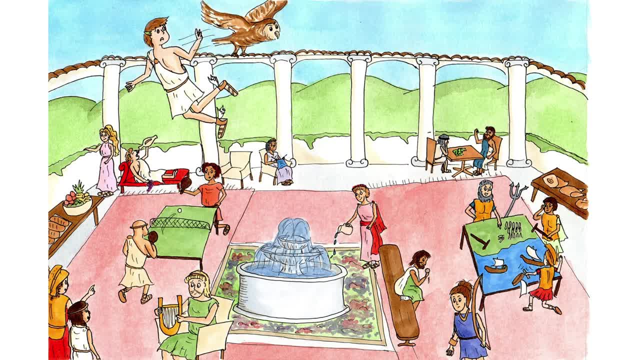 soldiers and ships. The man in red suddenly picked up a soldier and smashed it into one of the ships, crushing it to splinters. Your move, Poseidon. he roared. Delphi had no idea what was going on, And that's Artemis. 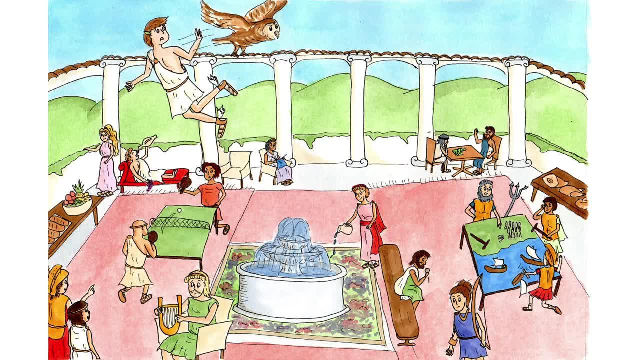 You probably know her. Athena nodded to a rather moody-looking dark-haired teenage girl who was dressed in furs and carrying a bow. She nodded at Delphi and she found herself nodding back: Hello, my angel. said a sweet-sounding voice. She looked round to see a beautiful young woman. 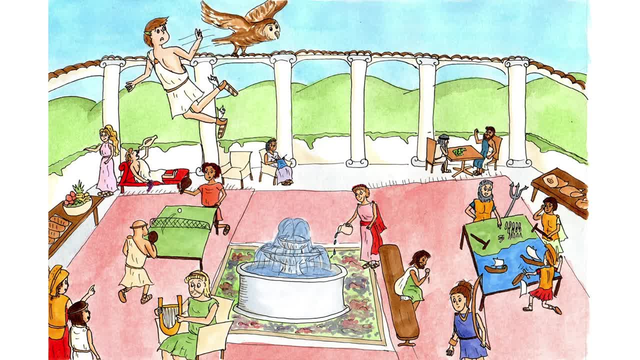 in front of her with long blonde hair and a pink dress. Can I help you at all? Is there someone who you'd like to get to know a little better? She gave Delphi a look that she didn't quite understand. She's not here to see you, Aphrodite, said Athena, pushing past her. 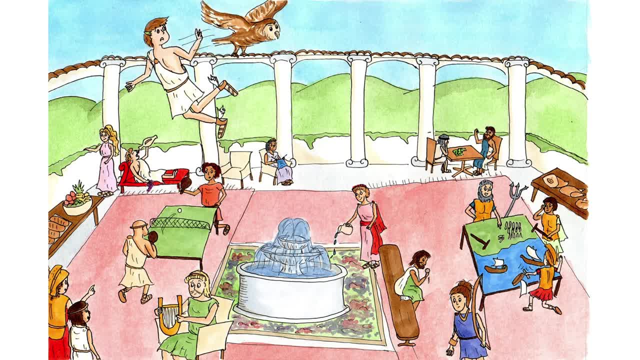 The blonde woman looked disappointed. Don't get involved with her dear. Nothing but trouble. Same for that one over there. She nodded in the direction of a curly-haired man who was holding a big jug of wine. When he saw her he looked panicked. 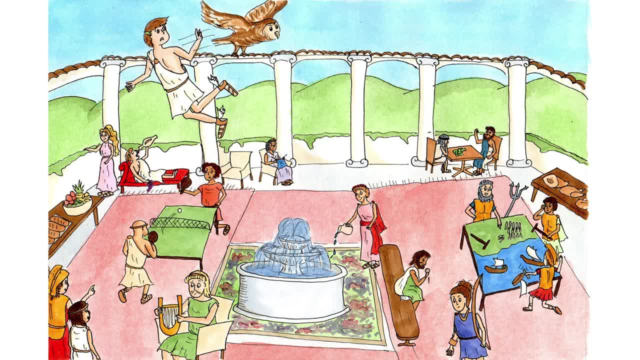 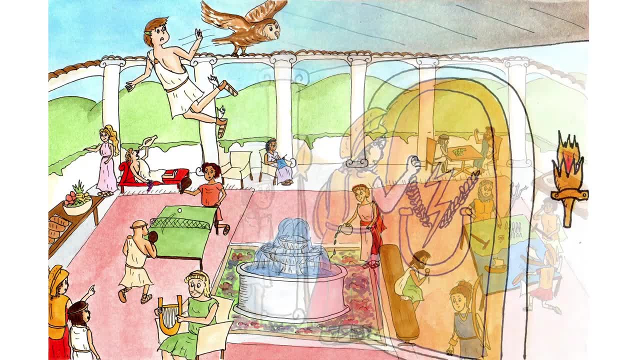 Dionysus. Delphi whispered: Um hello, girl, who I've never seen before, he said loudly. He gave her a look as if to say What the hell are you doing here? But Delphi just ignored him. Athena led her towards a big golden door at the back of the courtyard. 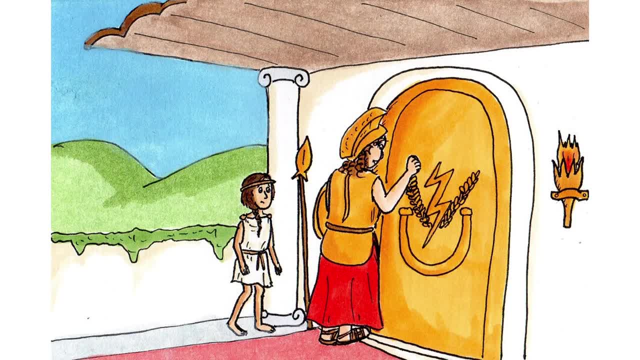 Zeus is probably just waking up now. Let's just go and make sure he's happy For visitors. you know what storm gods are like. first thing in the morning She knocked on the door. Yes, the voice boomed from inside. Good in, you go. 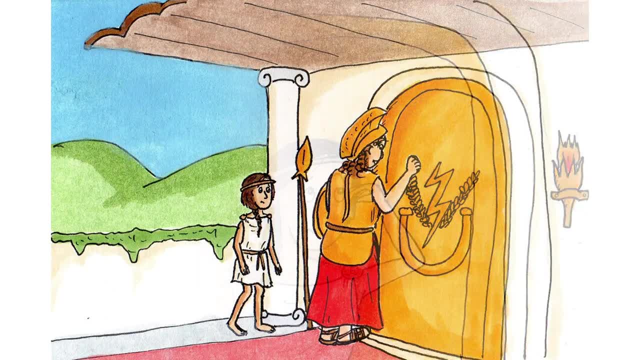 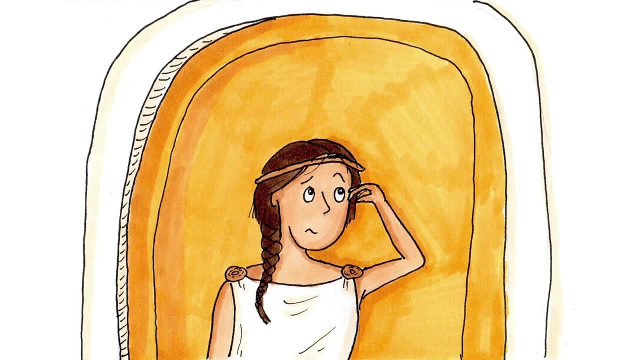 Athena opened the door and gave her a little push inside. Don't make him angry, dear. The door slammed behind her. Delphi took a deep breath. She could hardly take in what she had just seen. It wasn't quite what she was expecting. 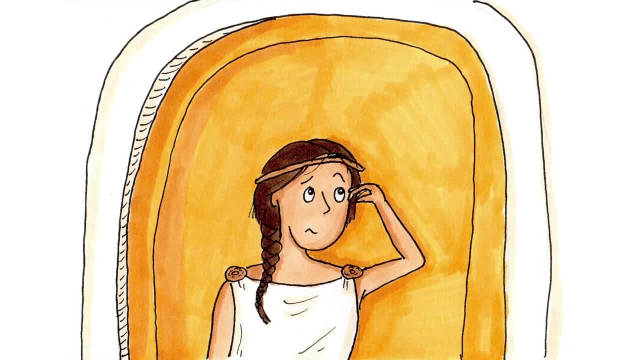 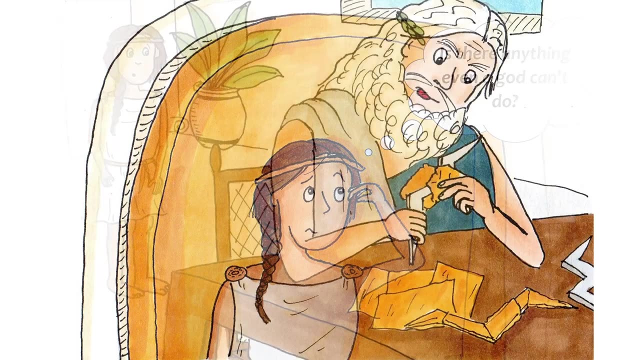 She was expecting all-powerful gods in an eternal paradise, not some kind of holiday camp for weirdos. Maybe the gods couldn't do everything they wanted, after all, Is there anything even a god can't do? Who is it Come here? 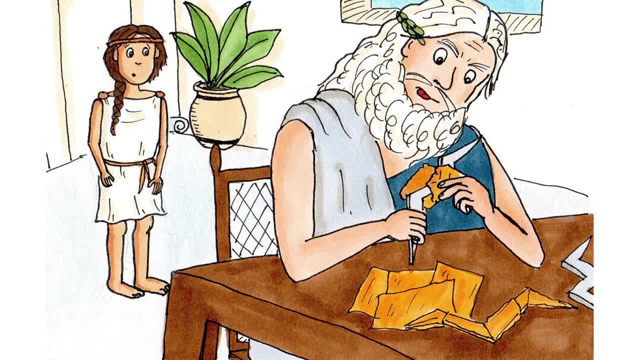 Delphi nervously stepped forward. Sitting at a table was a large old man with an enormous white beard. He had his back to her and appeared to be wrapping up some points of metal in what looked like yellow papyrus. Um, sorry to disturb you. you're um Zeus. 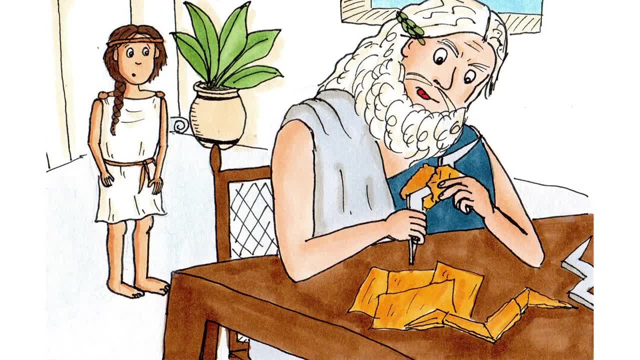 Delphi faltered. Yes, yes, What do you want? Zeus put down the thunderbolt he was making and looked up: Oh, you're not a god, are you? Uh, no, Thought not, but thought I'd better ask. It's hard to keep track of them all these days, There's so. 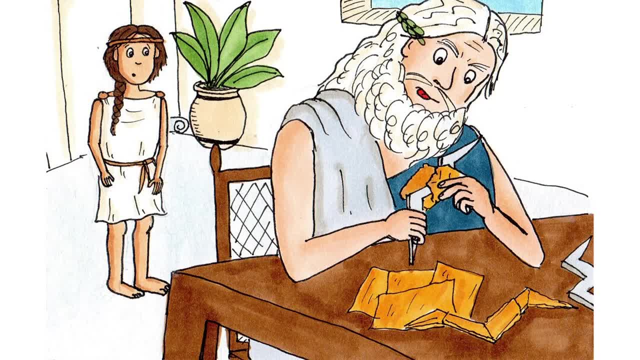 many. What's your name, girl? Zeus waved her to come closer. Delphi- Oh, it's the girl who wants to free Socrates, is it? Delphi nodded and tried to stop herself from asking how he knew. And I suppose you want me to free him, do you? 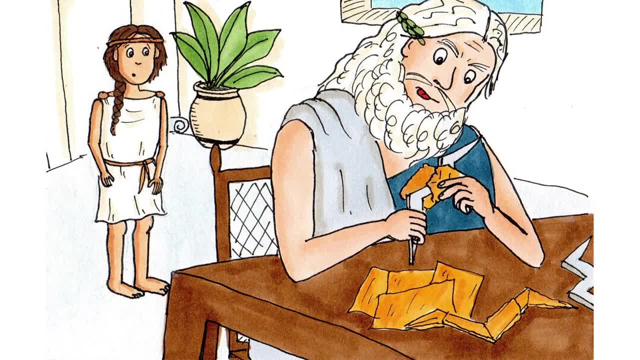 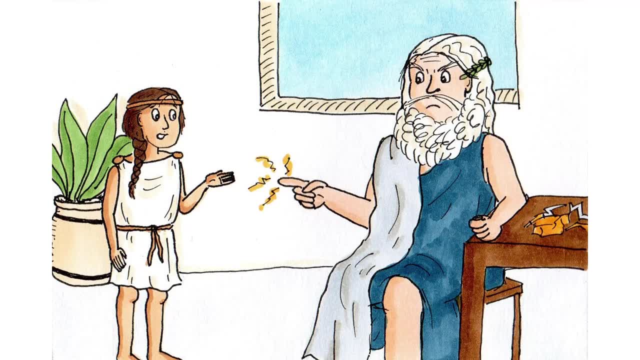 If you can. Delphi replied Then quickly realised this was not the right thing to say. What do you mean, if I can? Zeus shouted, thumping his fist on the table. All the thunderbolts he had made jumped up and sparked a little. 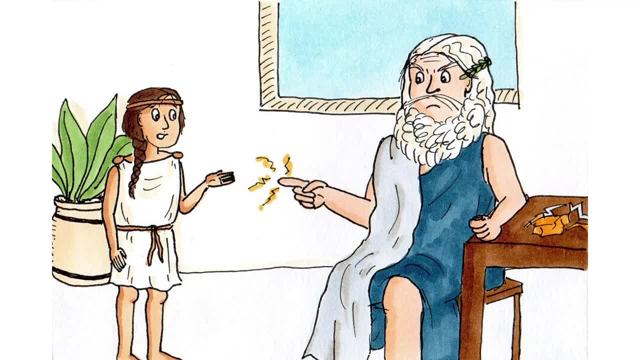 I'm the almighty father of the gods. I can do anything. Delphi waited for the thunderbolts to stop rattling. Can you, She asked. Of course I can, It's just I was thinking about it last night. There must be some things even gods can't do. 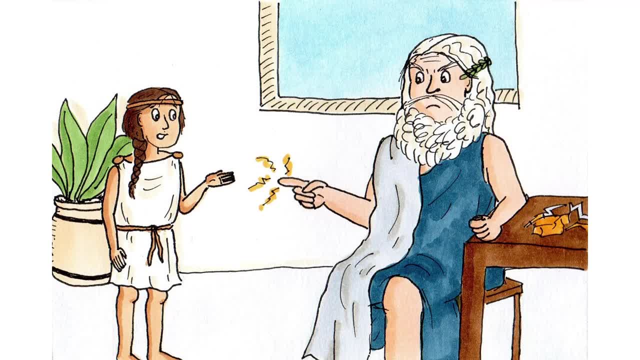 Delphi said: Oh really, You were thinking, were you? Zeus snapped. I don't like all this thinking People do nowadays. It was better when all you humans did was eat things and run around, Go on name something I can't do. 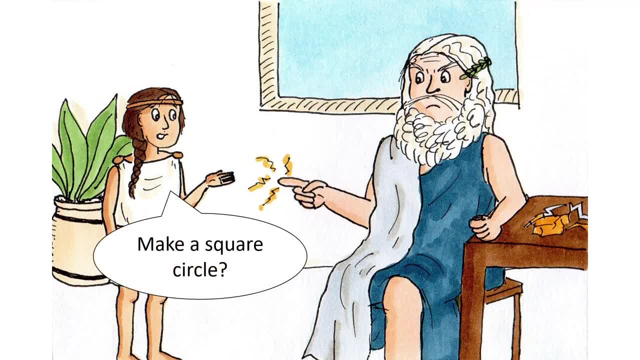 Delphi licked her lips. Make a square circle. Is Delphi right? Zeus hesitated. Well, or a loud silence? Delphi suggested That's impossible. Zeus declared throwing his hands up. There was a little snap of lightning from his hand. 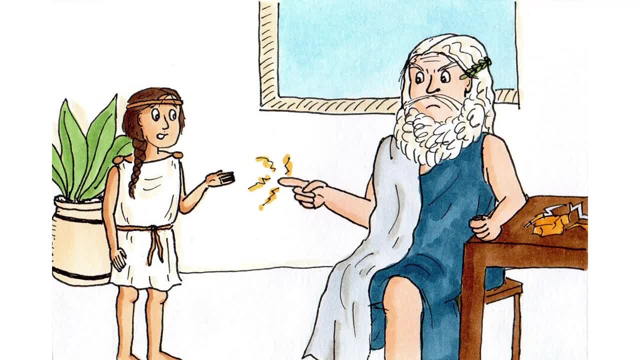 Delphi looked at his fingers, but he didn't seem to notice. Yeah, it is, Delphi, agreed. So you can't do impossible things. She hadn't intended to speak to Zeus like this, but somehow she couldn't quite help herself. 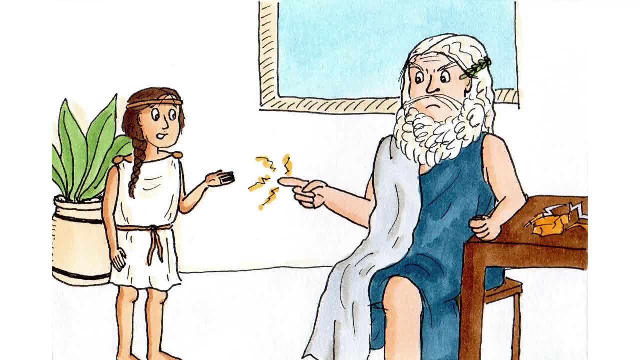 It must be all the philosophy she thought. Zeus gave her an annoyed stare. That doesn't count. You can't just say something that doesn't make sense and then declare I can't do it. Go on, name something that does make sense that I can't do. 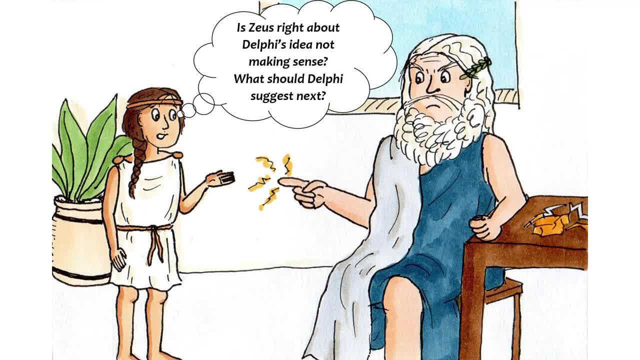 Is Zeus right about Delphi's idea not making sense. What should Delphi suggest next? What should Delphi suggest next? What should Delphi suggest next? Delphi thought about it, but not for very long, as it isn't a good idea to keep an angry god waiting. 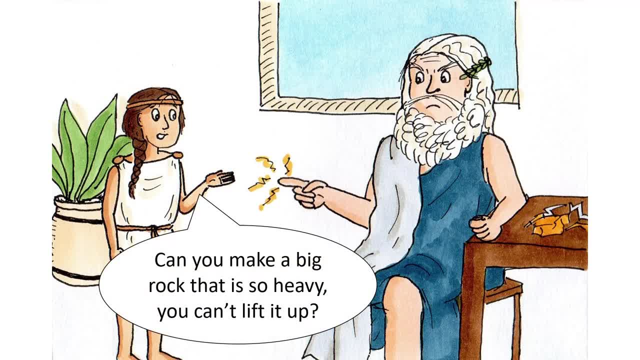 Can you make a big rock that is so heavy you can't lift it up? Delphi suggested: Of course I can. Zeus declared, He snapped his fingers. there was a flash of electricity and then there was a huge boulder taking up much of the room. 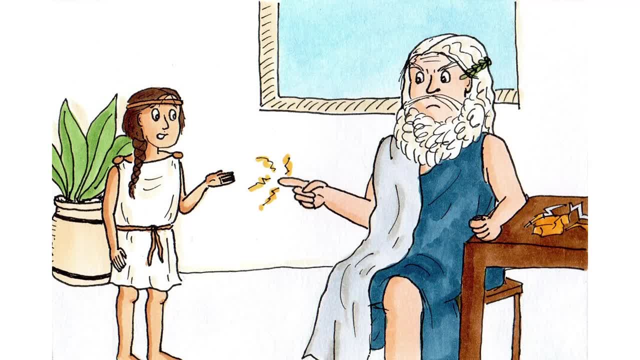 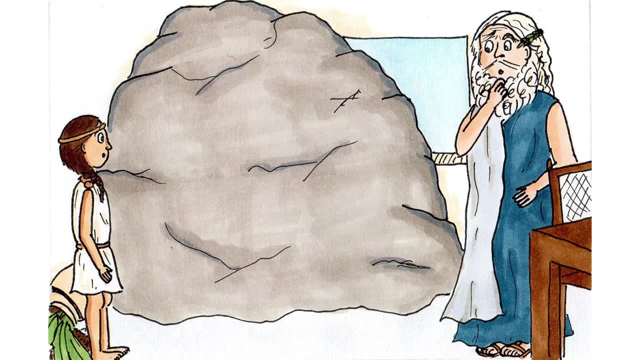 Delphi backed away from it nervously. It was three times higher than she was There. you go easy. Zeus stood up admiring his handiwork. Can you pick it up? Delphi asked quietly. Zeus laughed and started to wrap his hands around the rock. 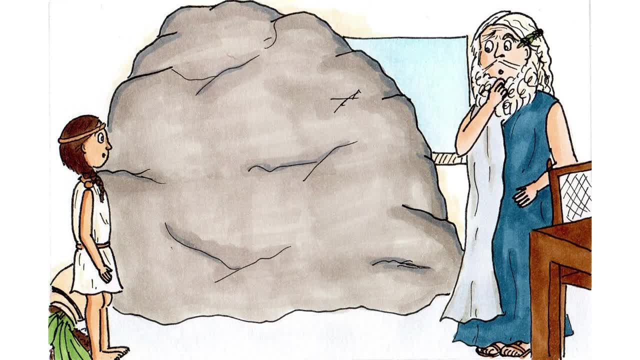 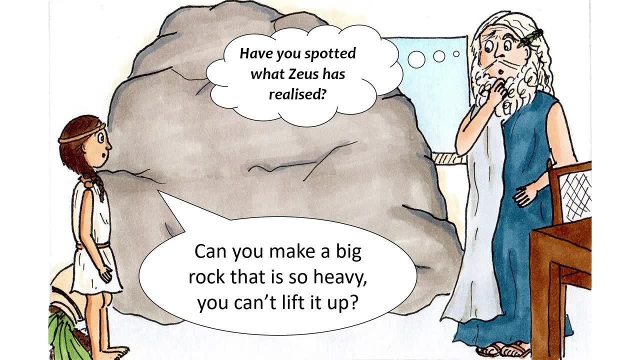 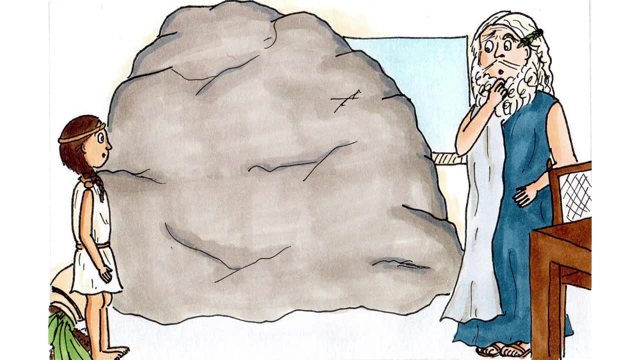 But then stopped. Wait a minute. he said: Have you spotted what Zeus has realised? Zeus stood up again and appeared to think This rock is meant to be so heavy I can't pick it up, right? So if I can't pick it up, then you win. 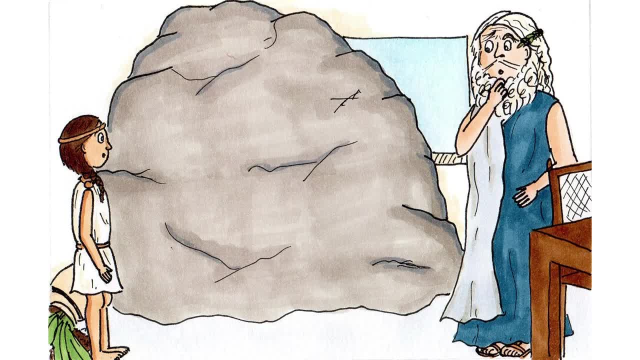 because I can't do it. but if I can pick it up, then I've failed to make a boulder. I can't pick up, then you win, because I can't do that. His forehead was creased in thought and then he: 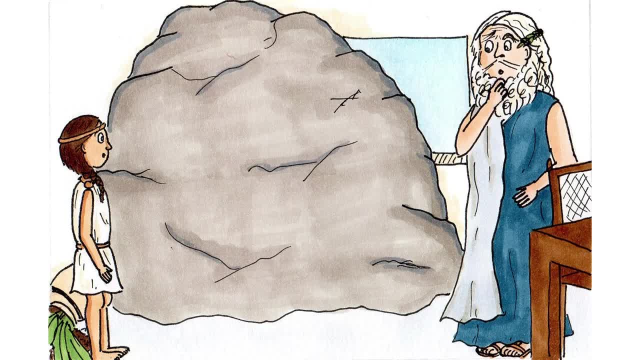 let out a shout: Oh damnation. Sparks flew off his beard. Delphi shrugged and tried to stop herself from smiling. Zeus sat back down, looked at her and then back to the giant rock. And now I've got a great big rock in my house that I can't get rid of, he yelled, thumping the table again. 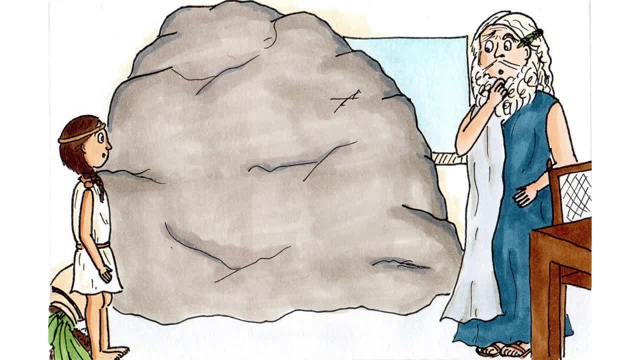 One of the thunderbolts exploded and Delphi leapt backwards. Perhaps she shouldn't have tried to be clever. I'm sorry. Delphi said I didn't mean to cause any trouble. I just wanted to know if you could free Socrates. Zeus slumped in his seat and appeared to take some deep breaths, That's all. 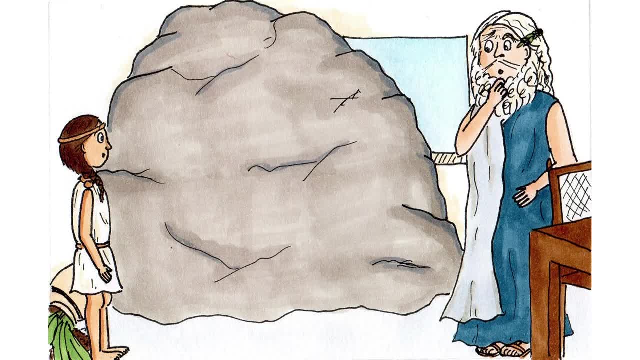 right, It's my fault. he muttered. I'll give the rock a few lightning bolts when you've gone. That'll do it. He smacked the boulder with his fist. It didn't move an inch. Ow, he added. 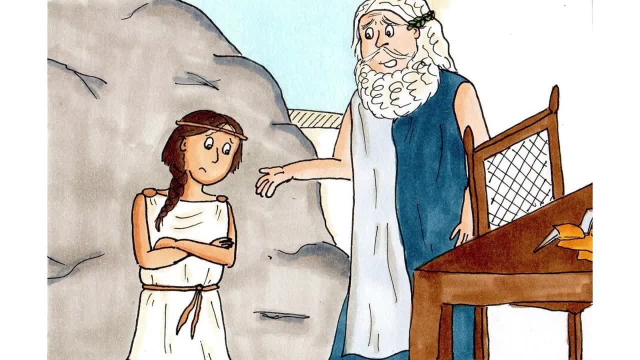 shaking his hand. But I bet you can free Socrates, can't you? Delphi asked. hopefully She was expecting him to agree, but to her surprise he looked even more depressed. Well, in a way, he replied. Delphi narrowed her eyes. What do you mean? Look, it's not all fun and games. 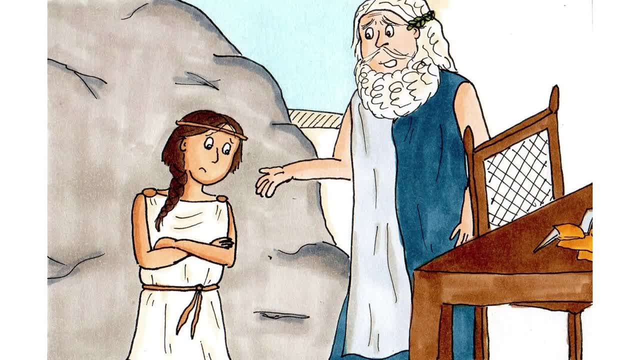 being a god. you know, Zeus moaned: Well, a lot of it is, But people always think we can do anything we like, and we can't Not really Do. you know what free will is? Delphi hesitated for a moment. 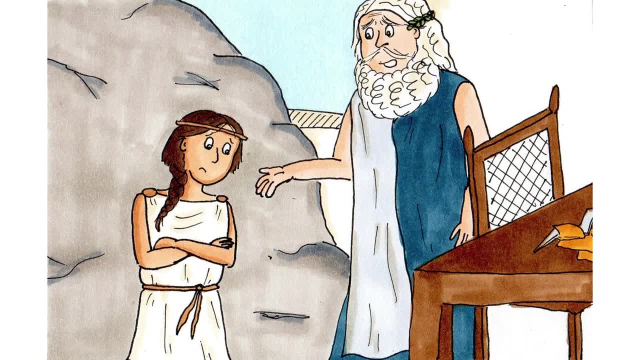 She wasn't sure she had heard that right Free will. Zeus repeated, catching her eye: Oh no, I don't know what that is. It's what all human beings have. It's the ability to think for yourself and decide for yourself, without anyone choosing for you. 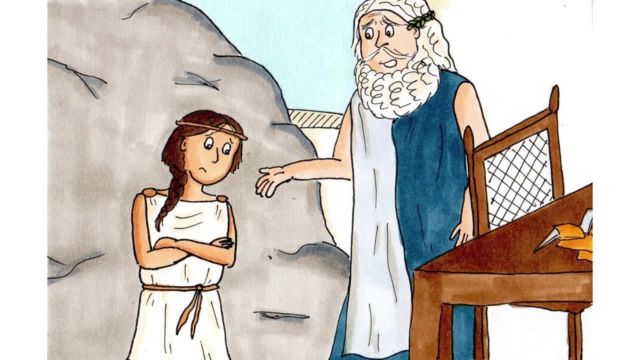 Delphi nodded. That sounded like something Socrates would believe in. Well, to get Socrates out of jail, I'd have to change the mind of all the guards and half the people in the city, wouldn't I? Otherwise they'd just lock him up again. I'd have to take away 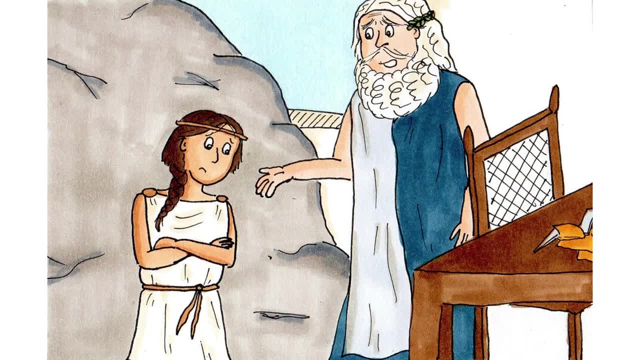 their free will to decide for themselves, wouldn't I? Zeus stared at her, I suppose so, And even Socrates himself? I'd have to decide for him, wouldn't I? I'd have to decide he can leave jail and stop being such an irritating, boring old duffer who goes around annoying people. 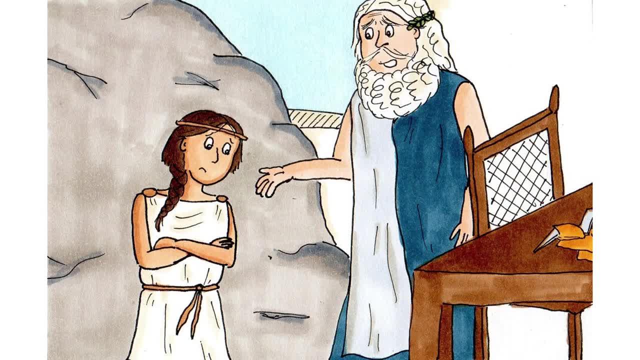 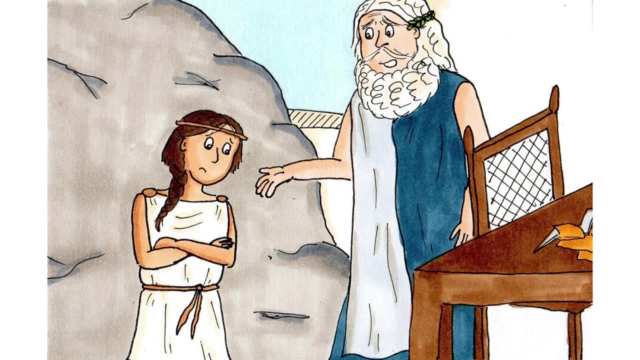 Otherwise he'd just get locked up again. I'd have to decide for him. Zeus repeated: Would he be free if I decided for him? Delphi understood what he meant and shook her head. Her heart was sinking. So you can't free him, because if you did, you'd be deciding for him, So then he wouldn't be free. 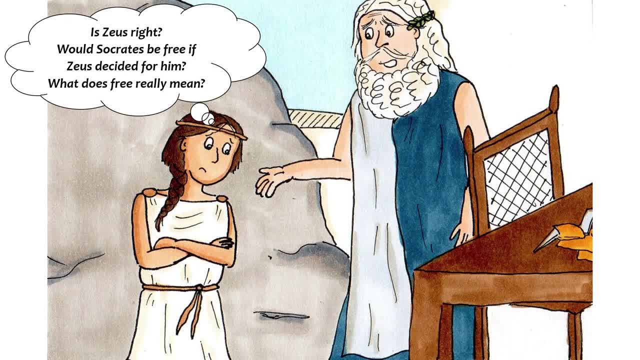 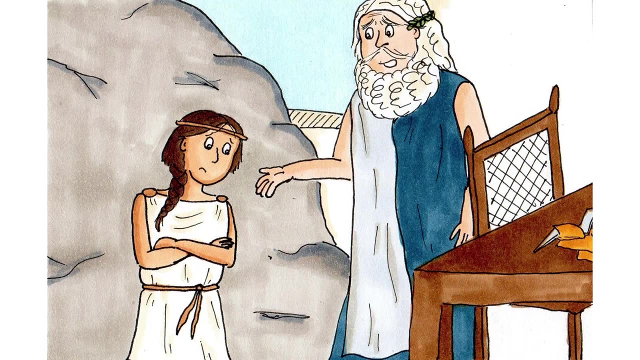 Is Zeus right? Would Socrates be free if Zeus decided for him? What does free really mean? Delphi smacked her fist on the table. Oh damnation. Zeus carefully moved some of the lightning bolts away from her, So you really can't do anything. Delphi asked. 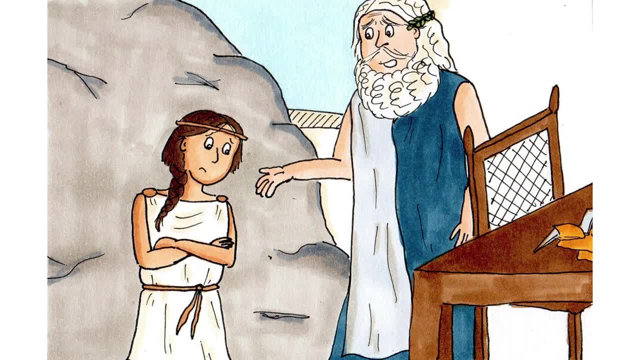 That's the problem with free will. Zeus replied sadly: Never should have given you humans that Ever since then. there's not much we can do with you. Come on, let's get you home. You're going to wake up soon. Zeus stood up and they squeezed past the boulder and back to the courtyard with. 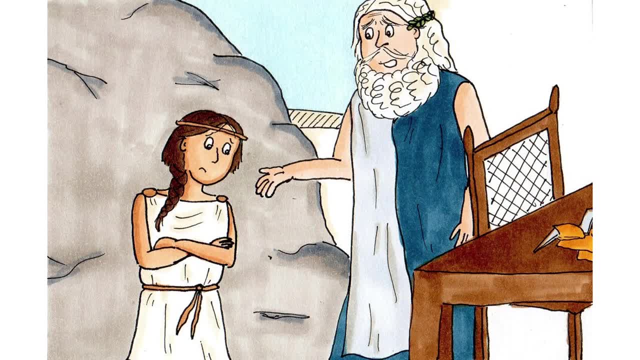 the other gods. Delphi felt utterly dejected. It felt like the whole universe was against her. If even the gods were to do anything to her, she'd have to do it, She'd have to do it, She'd have to do it. 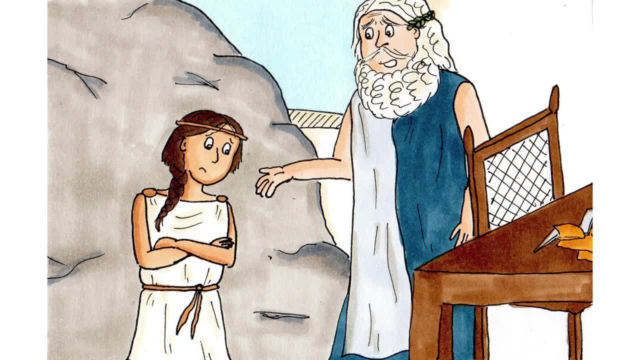 If even the gods couldn't free Socrates, then what could she possibly do about it? Now? now there's no need for a face like that. Athena said cheerfully when Zeus led her back to her. Zeus, what did you say to her? Nothing, Zeus replied guiltily. He turned to Delphi. 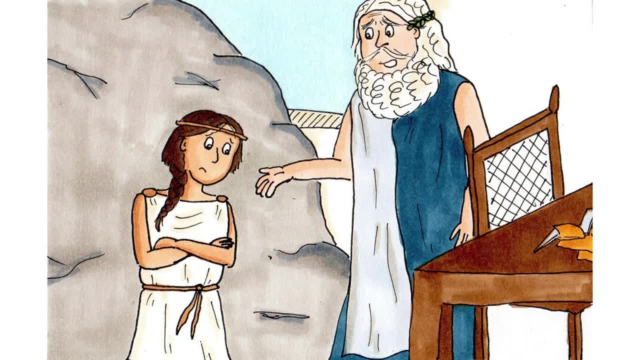 Tough luck, kid. Now, if you'll excuse me, I've got an immovable boulder to move. Zeus marched back through the golden door and shut it behind him. A few seconds later, Delphi could hear the rumble of thunder and muffled swearing from behind it. 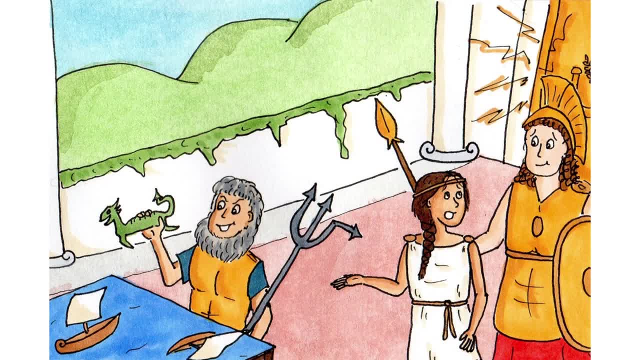 Did you not manage to free your Socrates? then Athena asked. as she led Delphi back through the courtyard, The other gods ignored her. Most of them were watching the game that the armored men were playing. Poseidon had just crushed a little model town with a sea monster There. I told you I'd get. 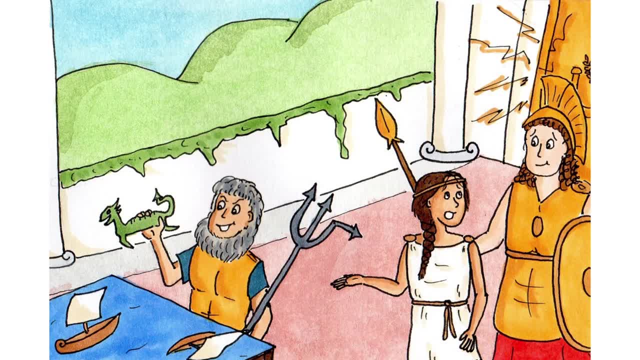 Atlantis. The spectators gave a mix of cheers and groans. Delphi looked back at Athena. No, it's to do with free will, apparently. Oh yes, Athena agreed. Always tricky that, Mind you, you've got a jolly good one of those, you know What. 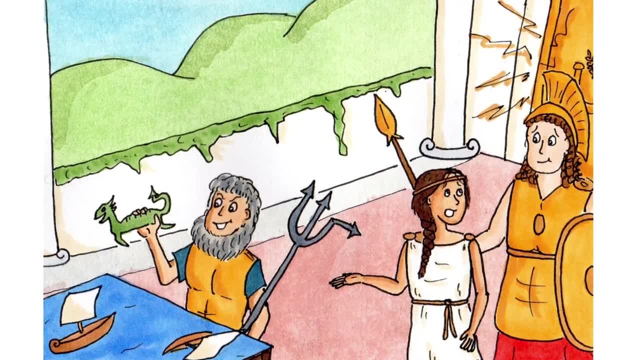 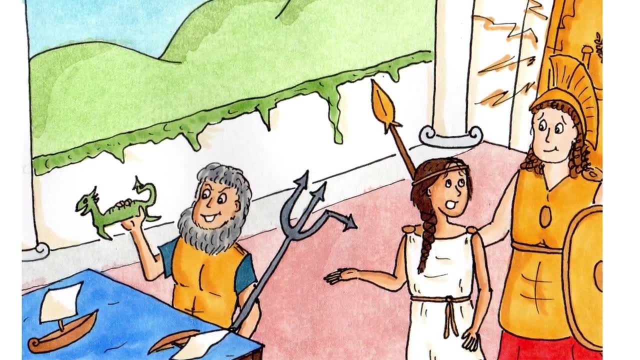 Athena stopped when they got to the edge of the courtyard and looked down at her. Just because Zeus can't do anything about free will, it doesn't mean that you can't. you know, You seem a very capable young woman. You did well with the invisibility ring and the bedroom. 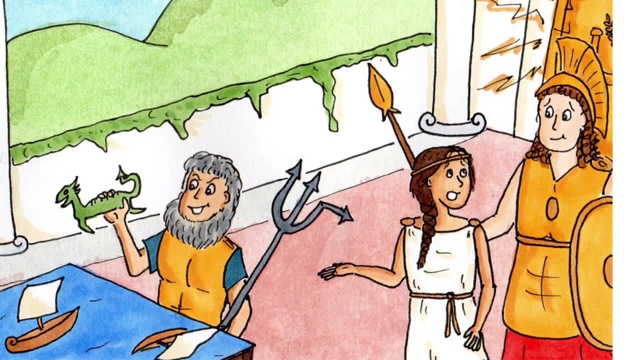 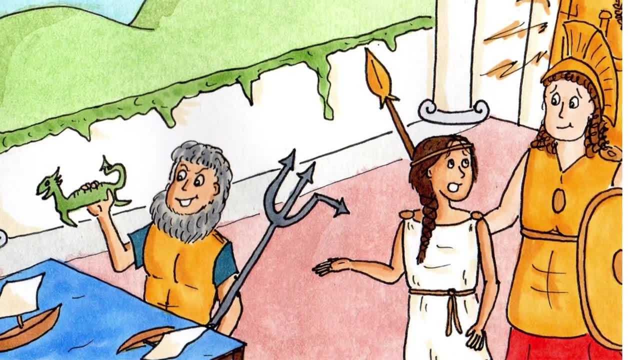 Delphi's mouth hung open. You know about all of that, Of course. You seem so set on becoming a philosopher that we thought we'd give you a helping hand. You know, give you some challenges that you could learn from, like Dionysus and his wish and the potions, You had us worried for a. 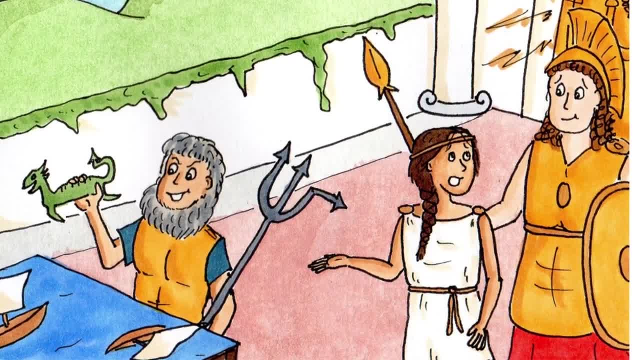 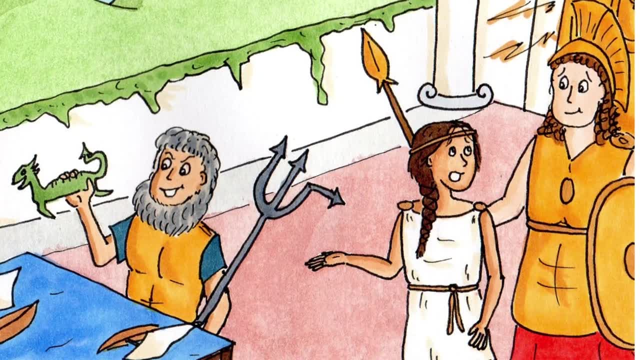 minute. with that one, Aphrodite was getting very excited. Delphi could hardly believe her ears. All of her recent strange experiences had come from the gods, as a kind of test. Don't look so hurt. We had your best interests at heart, my dear. 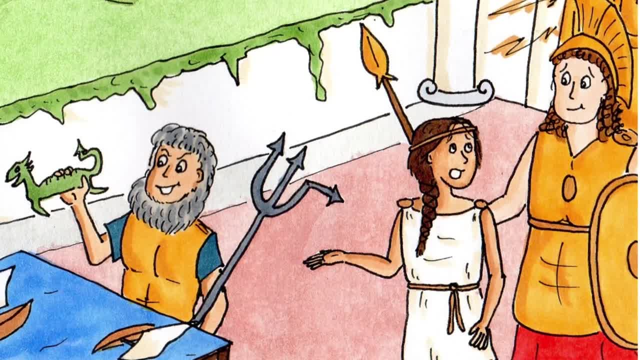 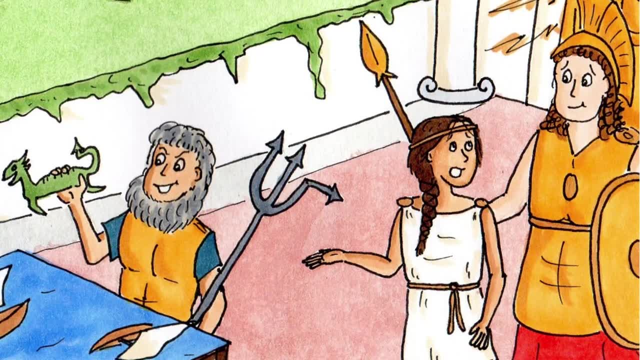 Athena said, putting her hand on her shoulder: The point is, you have learned from all that. You have learned to think for yourself, to ask questions and to use reason. You are a philosopher, Delphi. Delphi suddenly had a lump in her throat. She didn't know what to say. Athena looked her in. 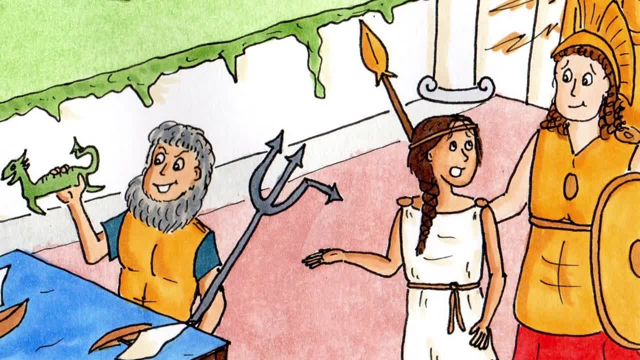 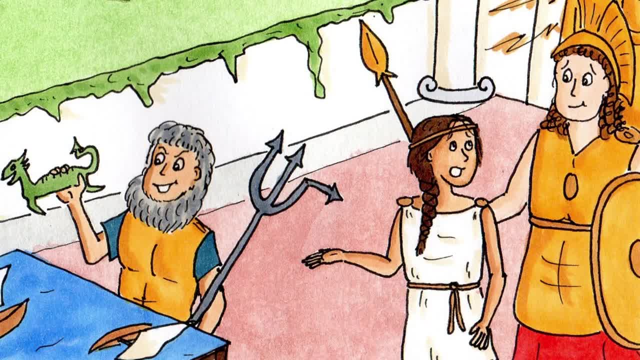 you up here. Delphi slowly nodded. She was a philosopher, She could do it. Athena stood up suddenly. Now, off you go, my dear, before you catch a chill from that cold marble floor you're sleeping on, and tell that young Mertis not to be such a big crybaby and to give my shield the 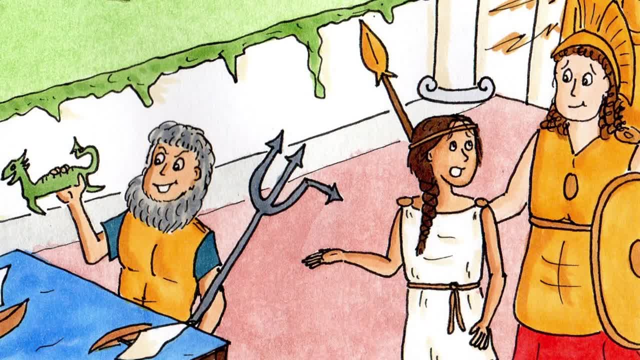 polish now and then. Uh, okay, thanks. Delphi walked away from the entrance to the courtyard watching as the room around her became darker and darker. She was falling back to sleep. When she woke up in the Parthenon the next morning she wasn't at. 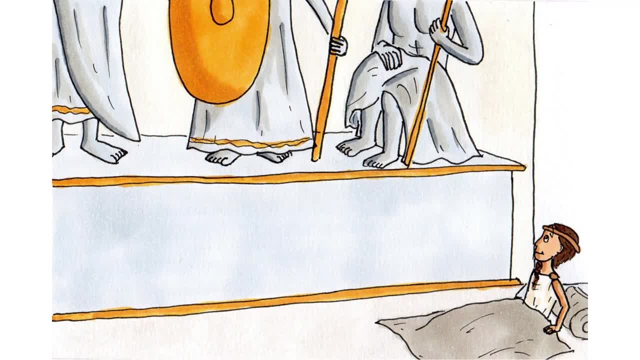 all sure how seriously to take her dream. She remembered it all clearly: the gods and goddesses, the boulder, the thunderbolts and Athena's words. She was a philosopher and, with the gods' help or not, she would make sure Socrates was free If the gods had decided that Delphi should try and 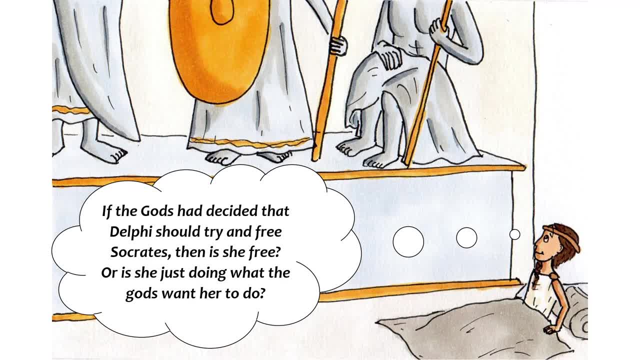 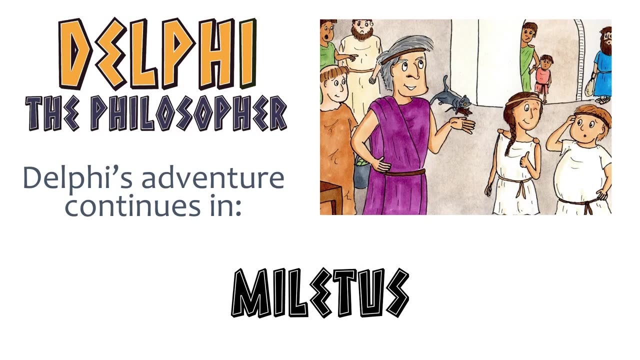 free Socrates then? is she free, Or is she just doing what the gods want her to do? How could she do what the gods want her to do? After a while, the voice in her mind seemed to be waiing. She had now changed and she was able to see clearly. 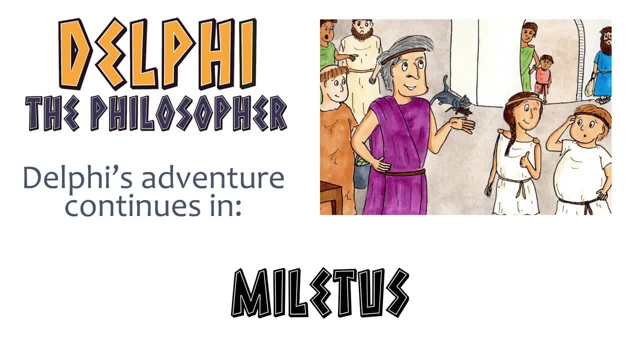 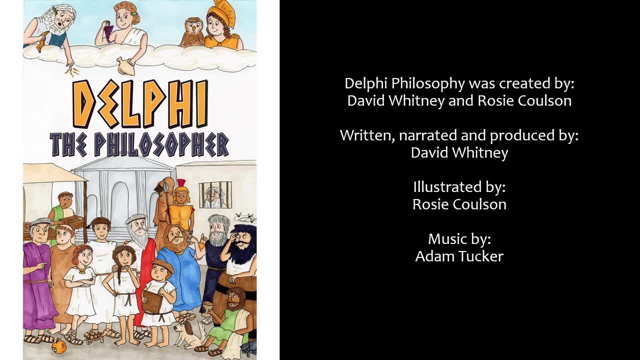 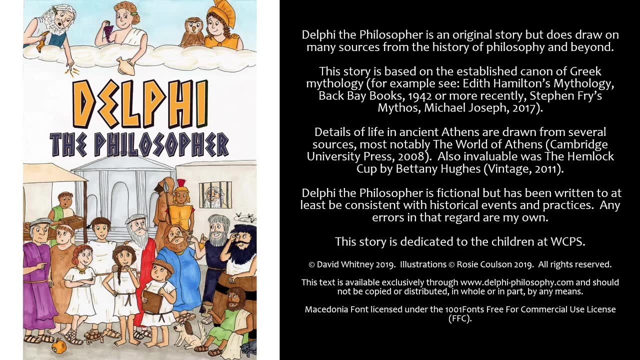 Who is she? She is Elisabeth. I am Elisabeth, I'm the goddess of the heavens And you're my god. You're Elisabeth, you're the goddess And you're the goddess of the heavens. No, you're the goddess of the heavens. Of course, Of course you.